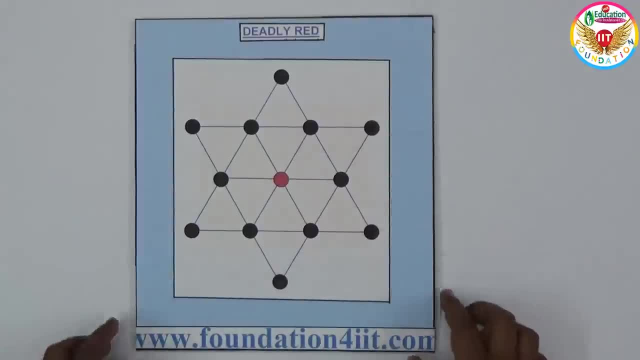 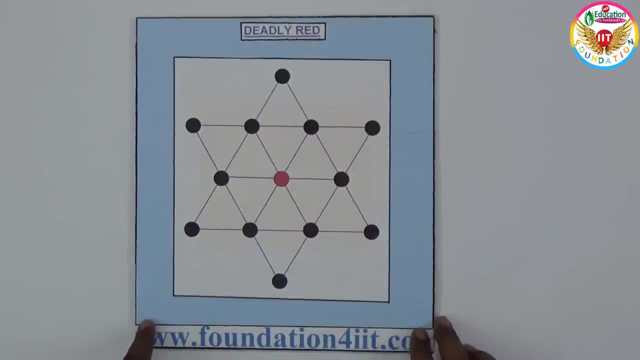 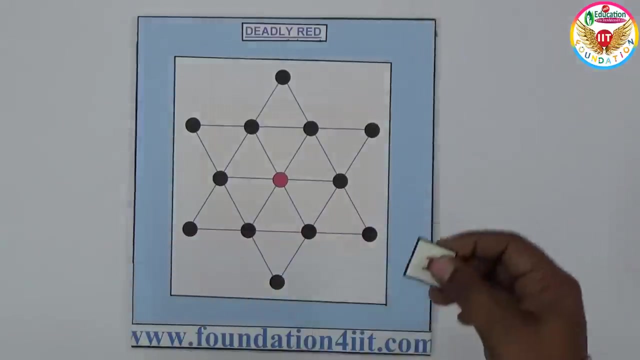 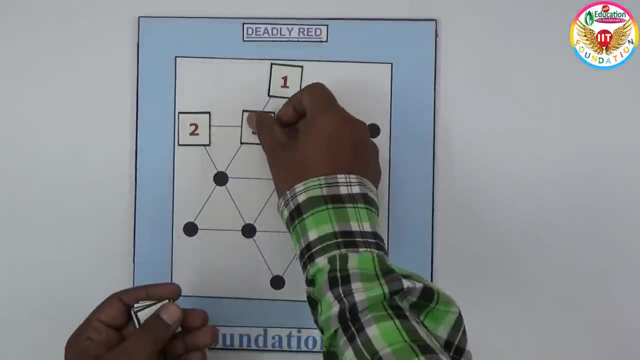 So one triangle and like this triangle you can join. So as it is, you can prepare. And middle one is red, So that's why you can call it deadly red. So I will show now what to do and how to play. So middle is red. Remaining all are 12, are there? So just 12 numbers. I took This 12 numbers. you can keep any place From all the black boxes, just you can keep 1,, 2,, 3.. So you can keep however you want. So 5,, 6,, 7,, 8,, 9,, 10.. 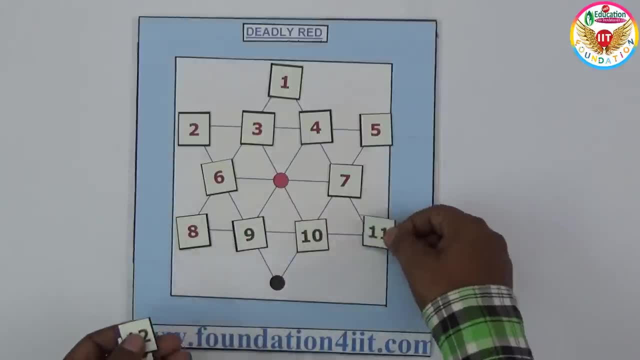 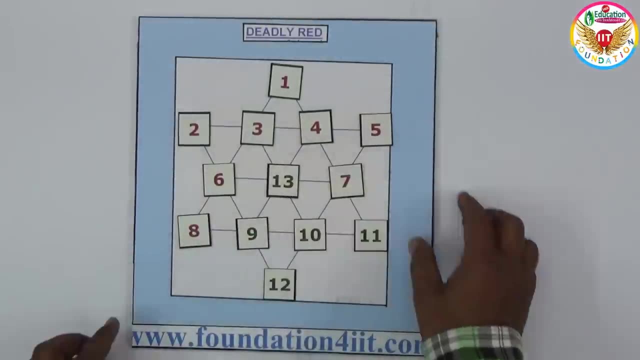 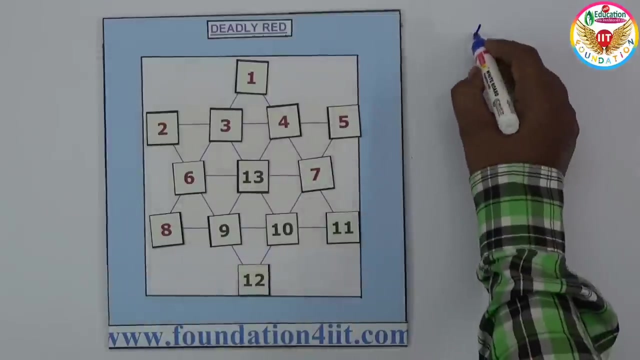 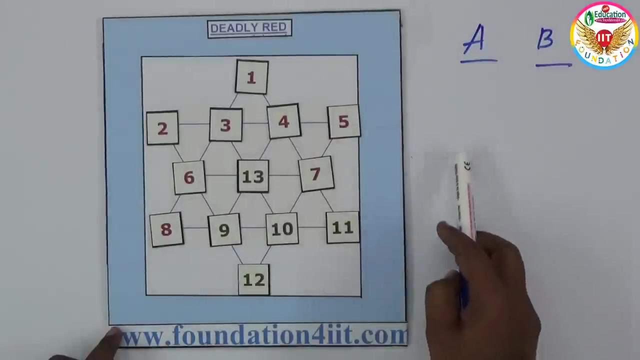 11, 12.. Ok, this, 12 numbers in this, 12 positions I kept, And middle is 13.. Now see how to play this. Actually, there are two players can play this. So say A and B, So A and B. Now the thing is, we need to take from any straight line any number of coins you can take from this, So not only numbers from 1 to 13.. 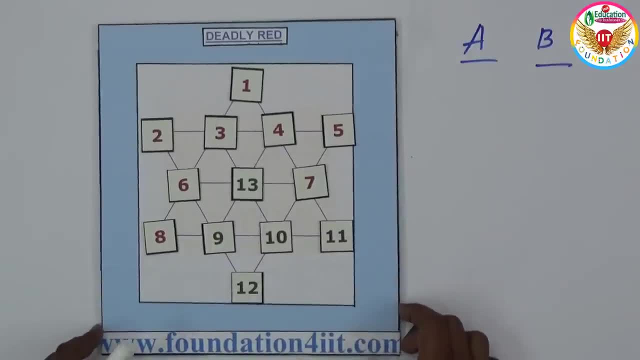 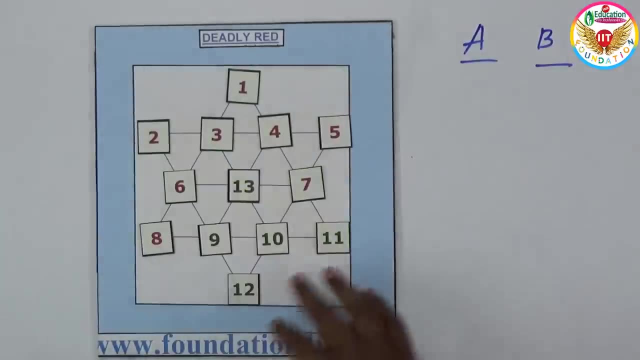 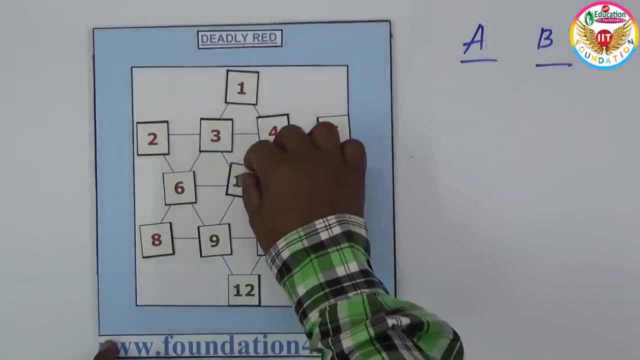 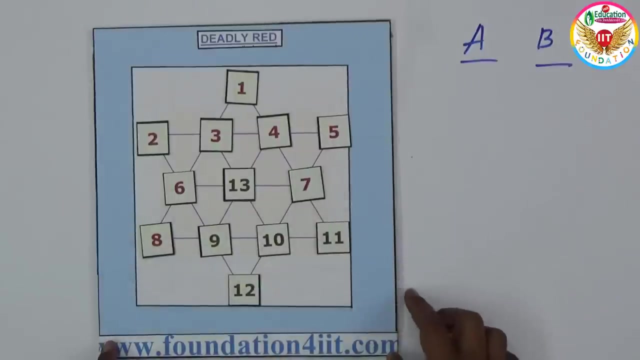 You can use normal coins or any marbles also in these places. Only thing is: we need to pick up from every straight line any numbers. So, for example, A wants to take some numbers in this, So who will take the last one is the loser. actually, That means you should give chance to opponent When all 12 are over. only last one should pick up. Last one should pick up at the ending. For example, A is taking from every straight line. only we should pick up some numbers. 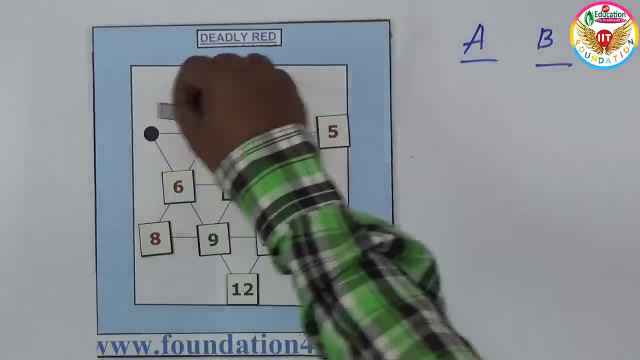 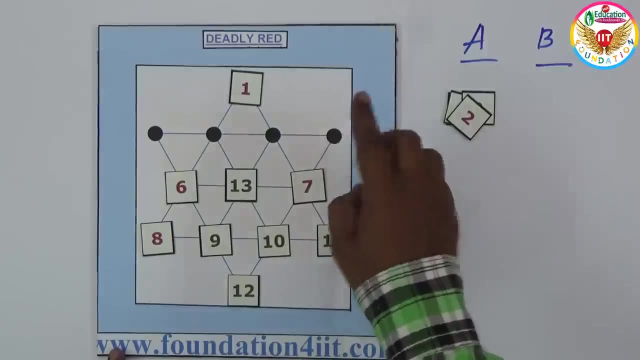 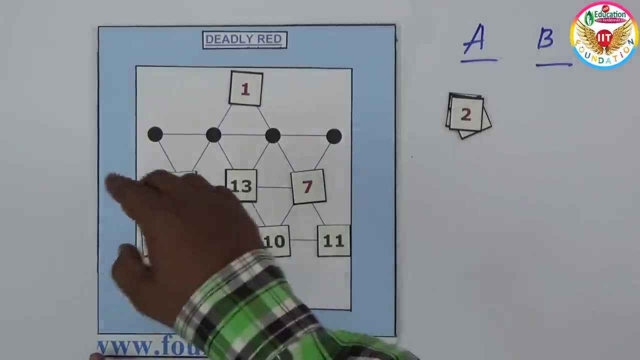 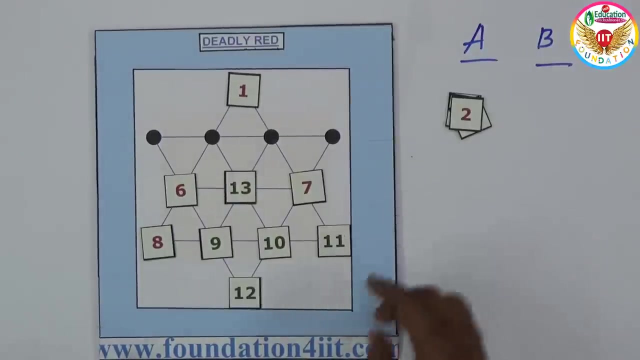 Ok, let us say A is taking all these numbers. Ok, 2,, 3,, 4,, 5.. So this is taken by A From this straight line, not only exactly 4, you can take even 2,, 1,, 3 or 4 also. But for every one chance we should take any number of coins or marbles from every straight line. only we should pick up: Ok, I have taken like this: Now chance for B, Now from this line or this line, middle one should not touch. 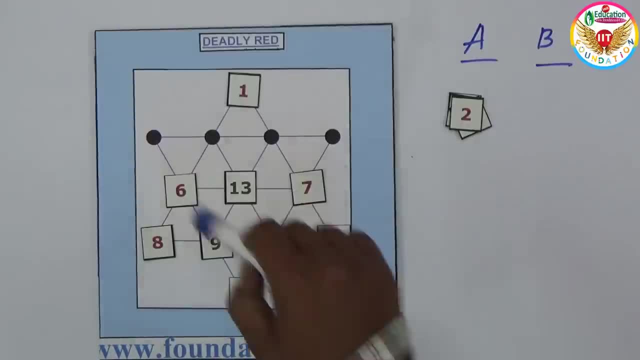 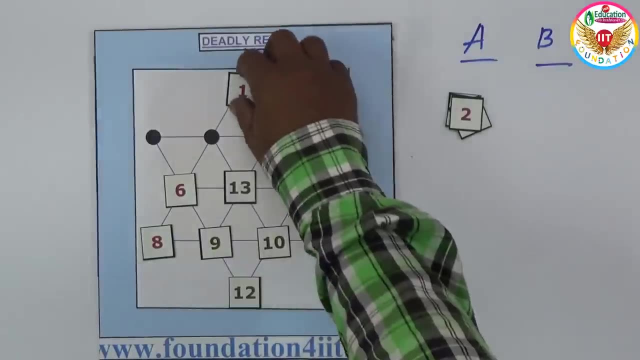 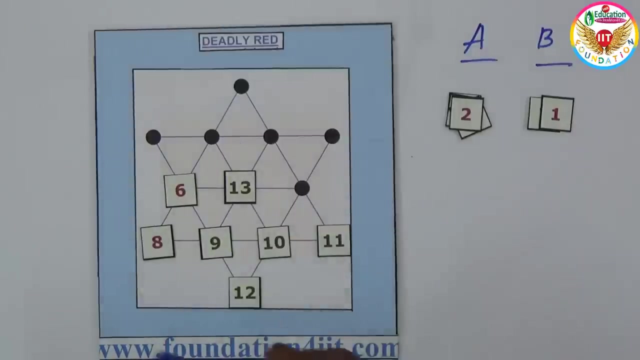 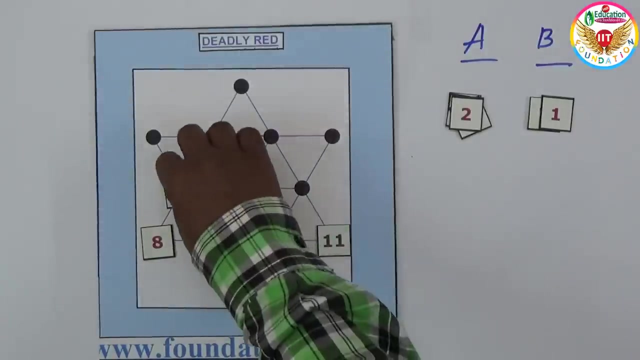 Ok, except middle line, Remaining straight lines only. we should pick up. Now, for example, chance for B, If you want to take from this, So you can take only, for example, 1 and 7.. Ok, imagine You took only 2.. Now again, chance for A. So from this remaining from every straight line only you should take. Ok, for example, A is taken from this complete line 6,, 9,, 12.. Ok, just take. 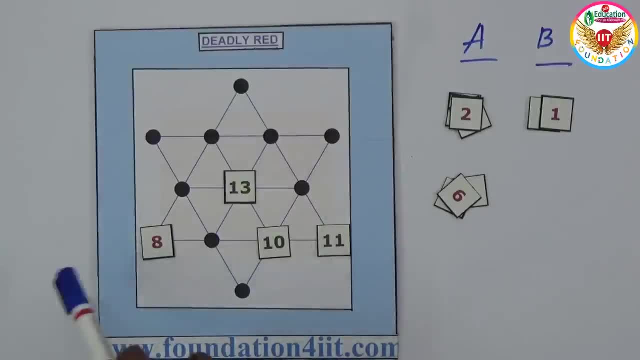 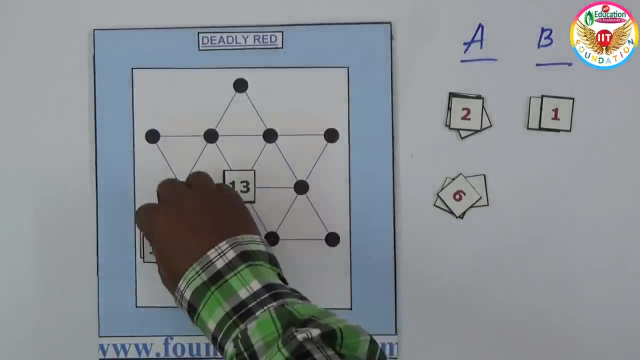 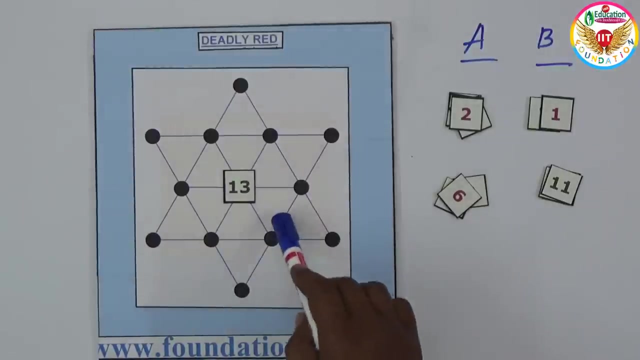 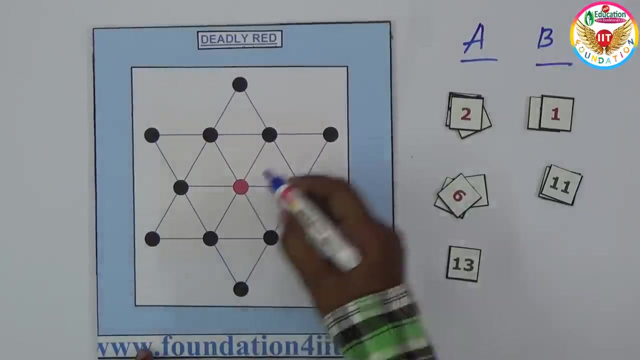 Now chance for B. Now B is this straight line, This complete straight line you can take, Because A can take only chances for 13 later. So it is B's winner. For example, B is taking these all straight line numbers. Now chance for A is only the middle. So, finally, who will give the chance for last number? Actually, they are the winner. Now B is taking 13.. So B is taking 13 because this is red. So he is the loser and B is the winner. So the concept was just only based on this. 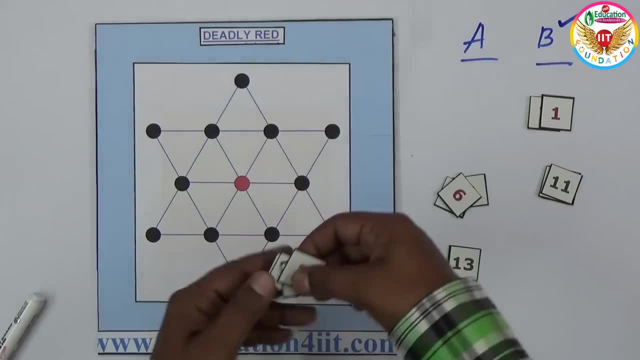 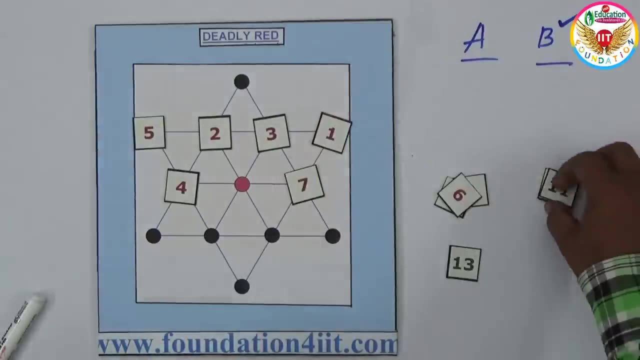 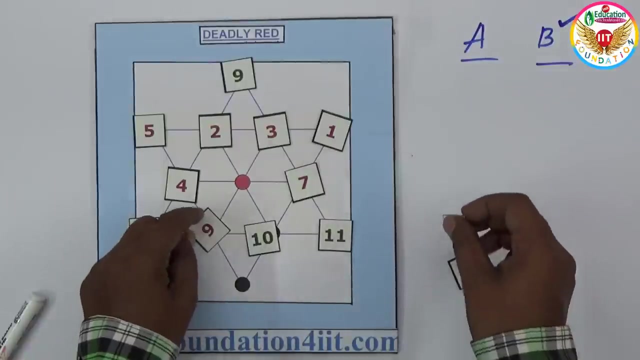 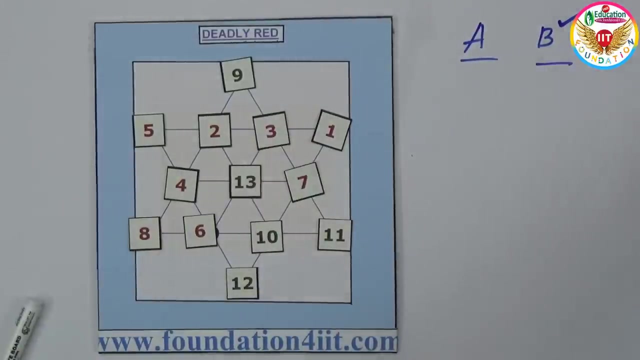 Ok, So you can do the same thing. You can take the lines from any straight line, only they should pick up, So you can keep anywhere, However, you can keep numbers, Or you can take the coins or some marbles, also in this place. The thing is you need to pick up one, Ok, No matter of exactly the same place. You can keep however you want Middle And middle one. just one more one thing you can keep. Ok. Now we need to think and play also this: For example, A is taking only from straight line. 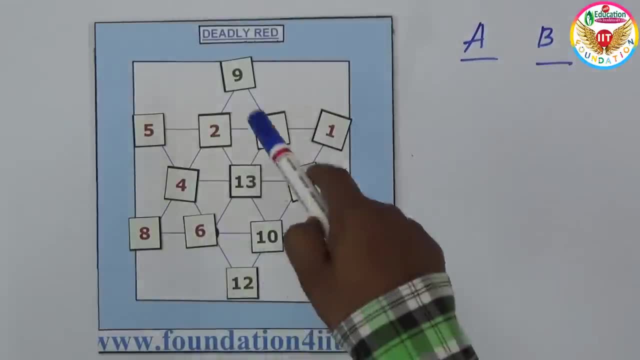 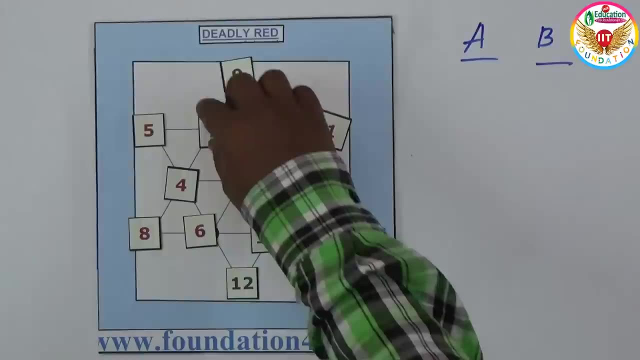 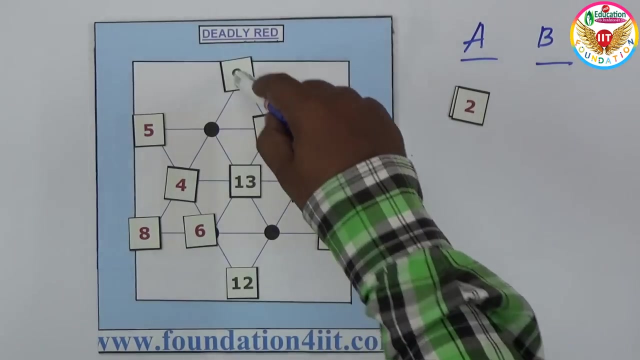 so not in zigzag way, because many straight lines are there. so from every straight line you should pick up. for example, this is straight line, now a is taking without touching middle. you can take this 2 and 10. okay, let's say a is taken like this: now chance for b. you need to think, for example, if 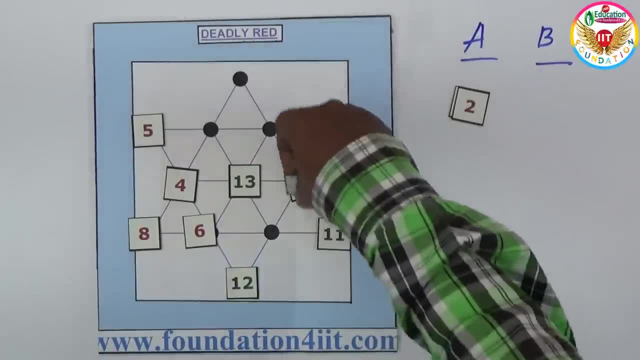 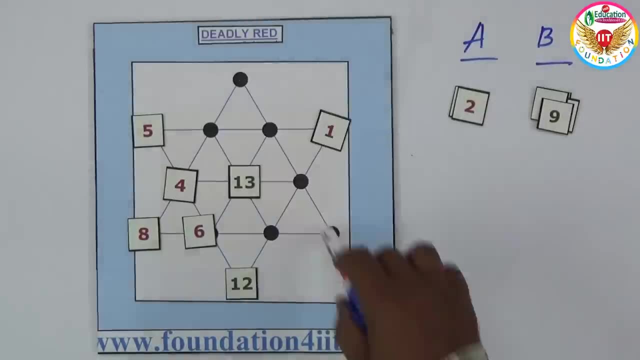 you take this complete line: 9, 3, 7, not only 4. you can take even 1, 2 or 3, even completely 4 also okay, b is taken. this complete. no chance for a. so a is taken. for example a if you take complete.